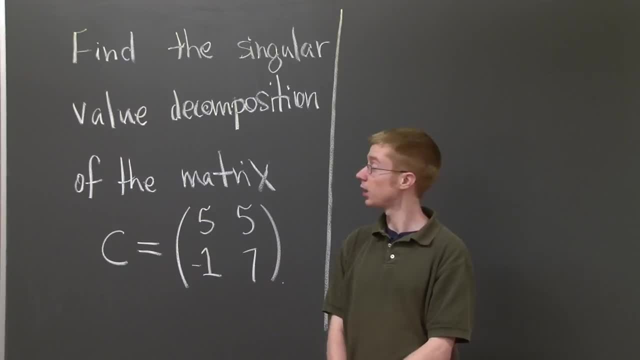 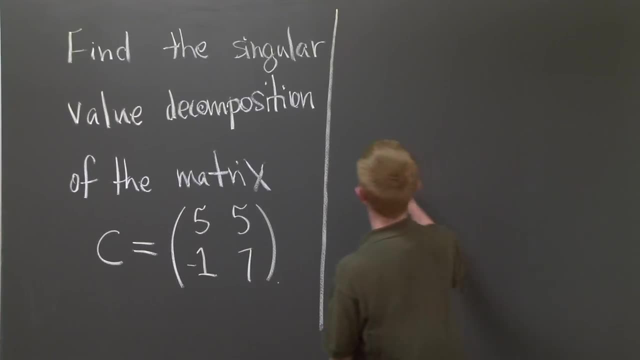 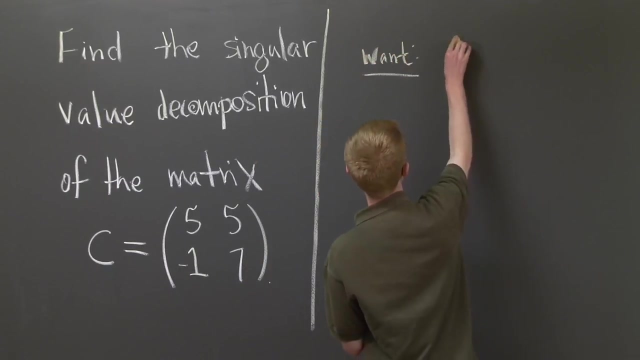 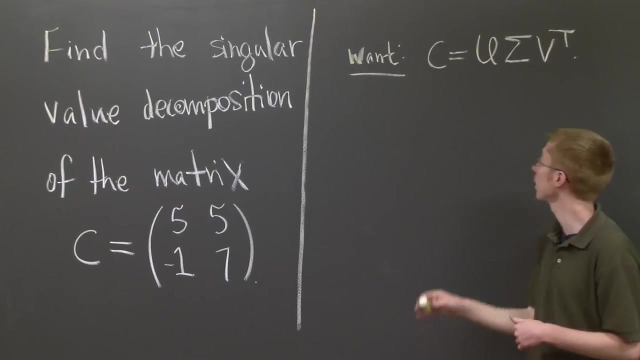 make a mistake, so you can never do enough examples of finding the SVD. So what does the SVD look like? What do we want to end up with? Well, we want a decomposition. C equals U sigma V transpose U and V are going to be orthogonal matrices. 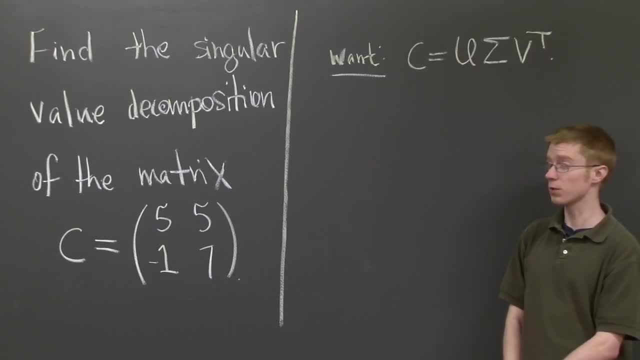 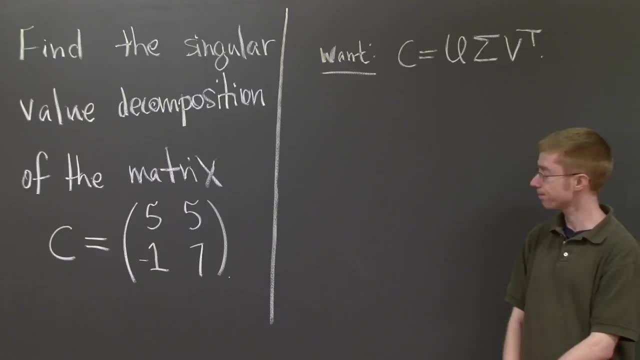 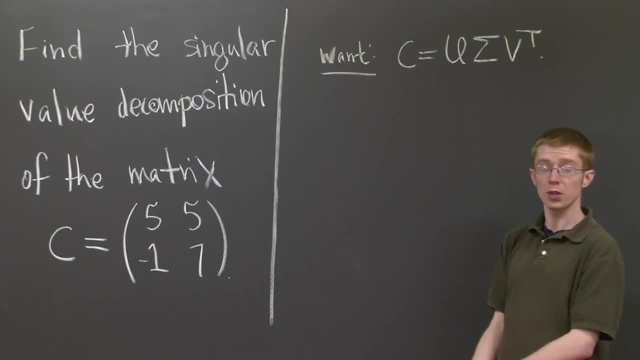 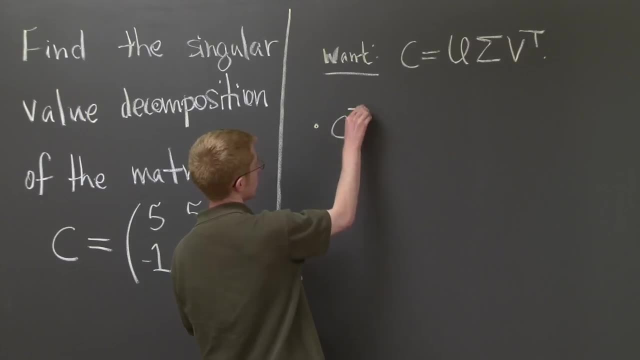 OK, good, So now how do we find this decomposition? Well, we need two equations. One is C transpose, C is equal to V sigma transpose, sigma V transpose. And you get this just by plugging in C transpose, C here and noticing that U transpose, U is 1, since U. 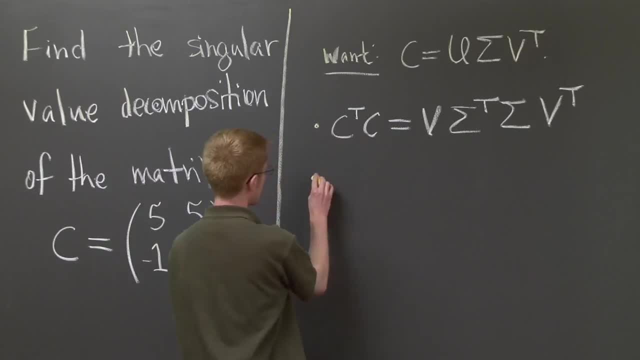 is an orthogonal matrix And the second equation is just noticing that V transpose is V inverse, and moving it to the other side of the equation, which is C, V equals U sigma. OK, so these are the two equations we need to use to find V sigma and U. OK, so let's start. 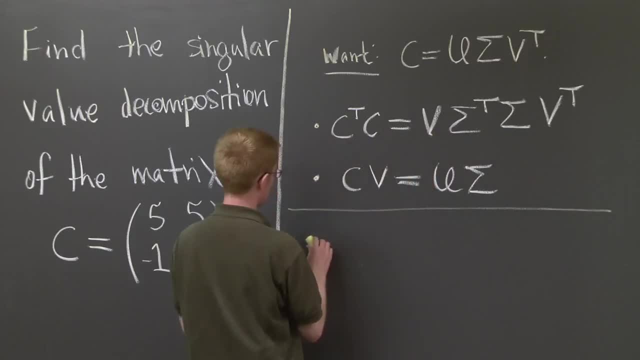 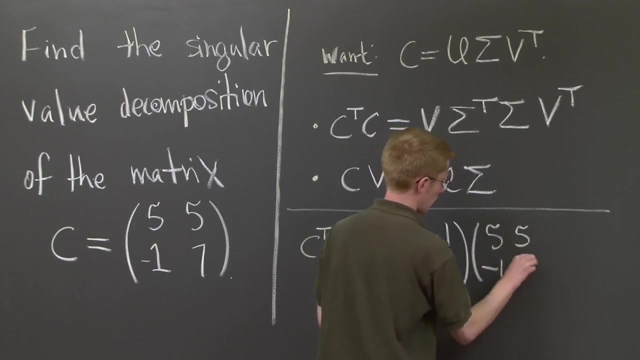 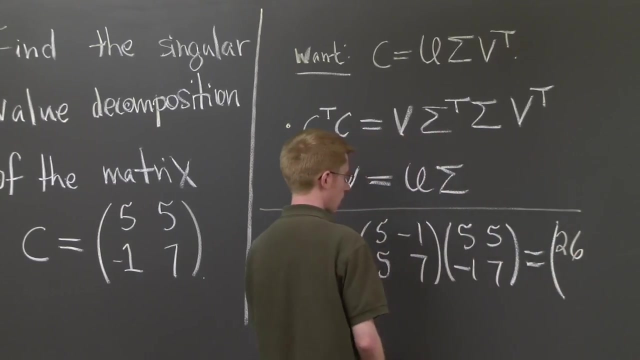 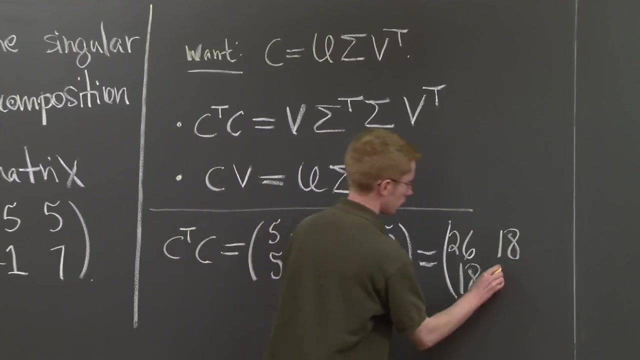 with the first one. Let's compute: C transpose C. So C transpose C. what is that? Well, if you compute, we'll get a 26,, an 18,, an 18, and a 16. So we'll get a 74.. 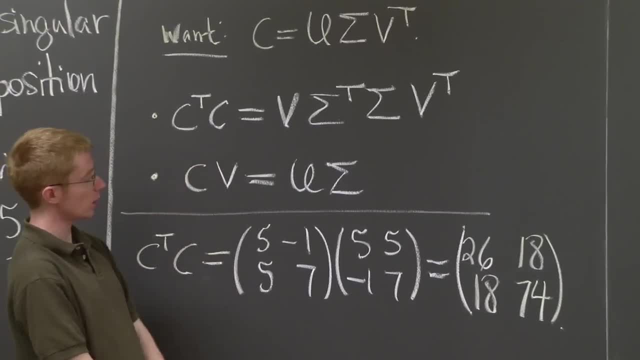 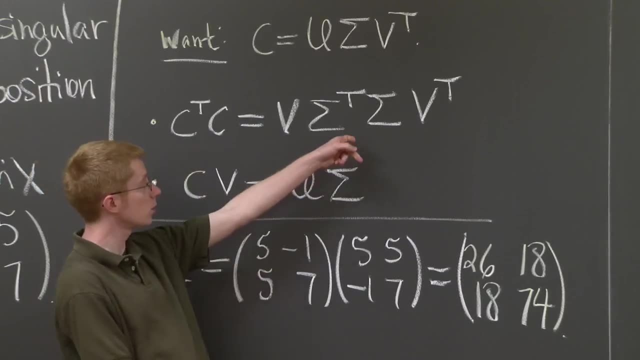 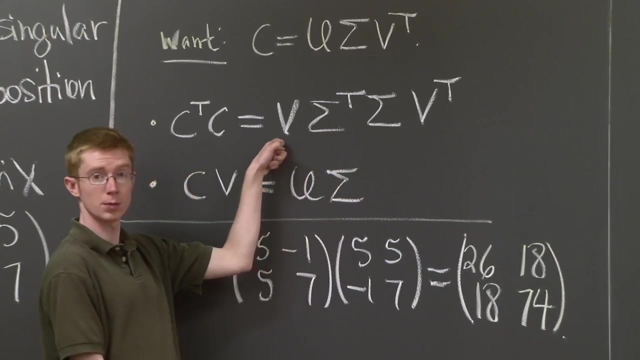 Great. Now what you notice about this equation is: this is just a diagonalization of C- transpose C. So we need to find the eigenvalues- Those will be the entries of sigma, transpose sigma- and the eigenvectors, which will be the columns of a, V. OK, good, 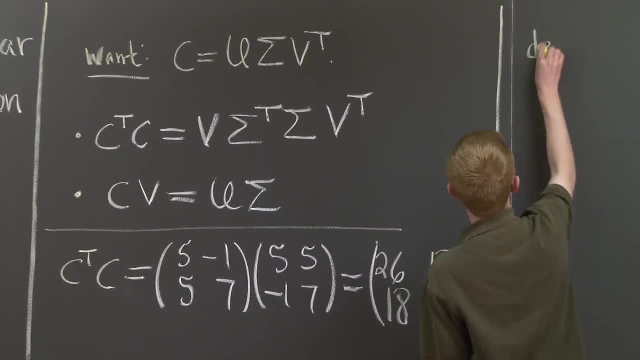 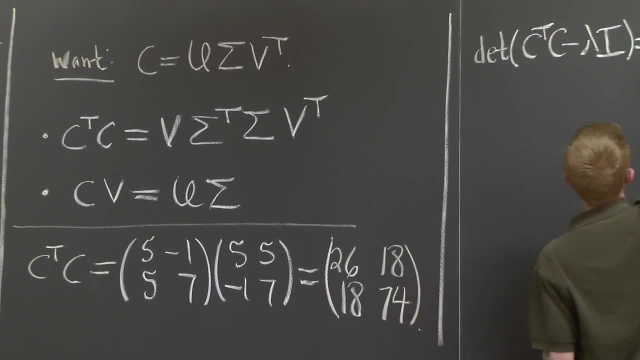 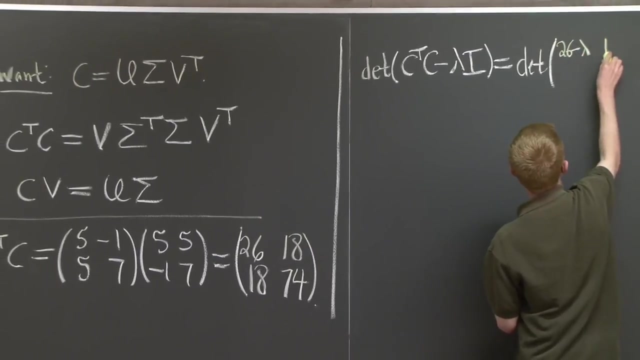 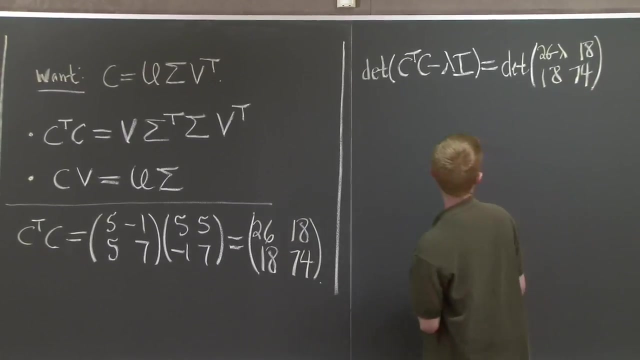 So how do we find those? Well, we look at the determinant. We look at the determinant of C. transpose C minus lambda times the identity, which is the determinant of 26 minus lambda, 18,, 18, and 74.. OK, 74 minus lambda, thank you. 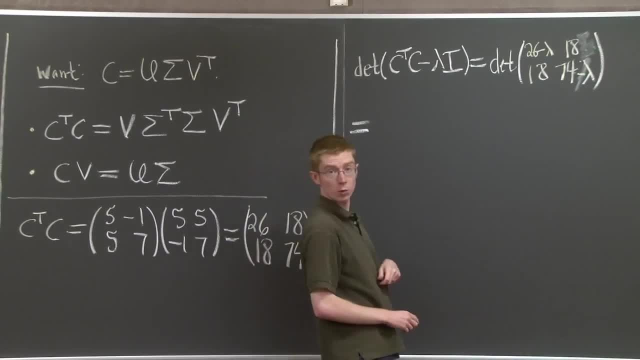 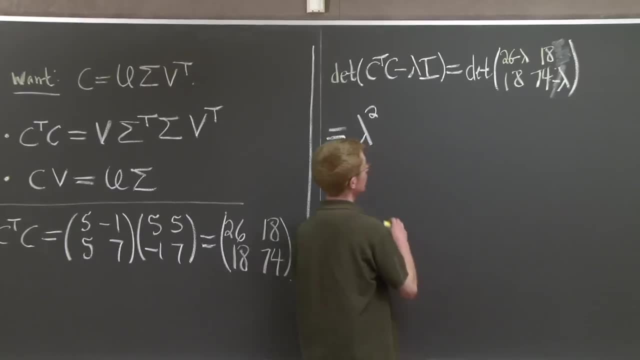 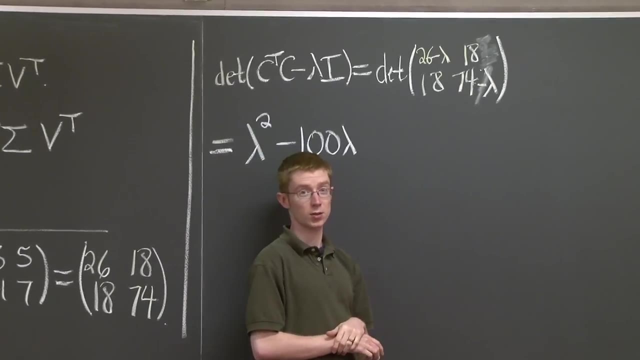 Good, OK, and what is that polynomial? Well, we get a lambda squared. Note that 26 plus 74 is 100, so minus 100 lambda. And I'll let you do 26 times 74 minus 18 squared, on your own. 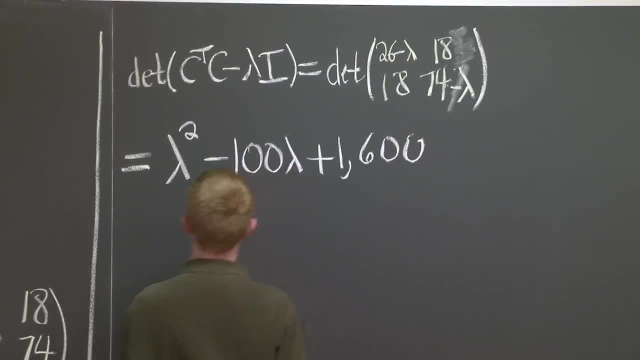 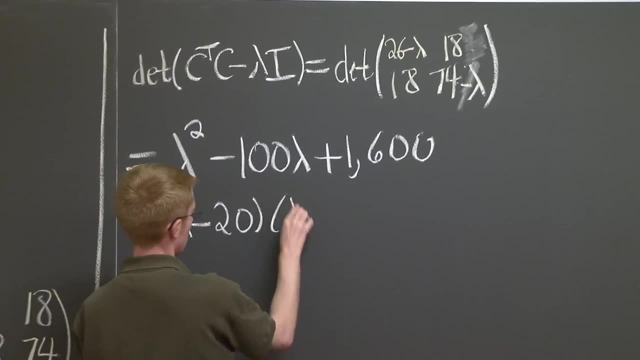 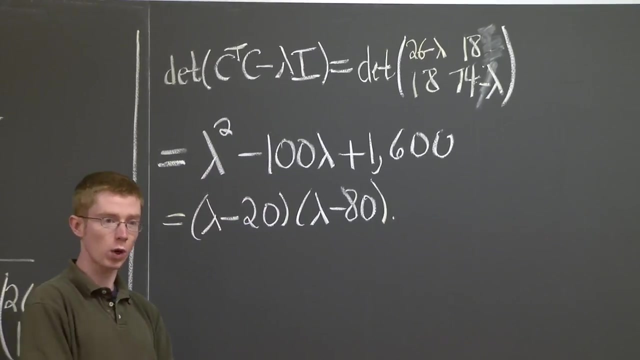 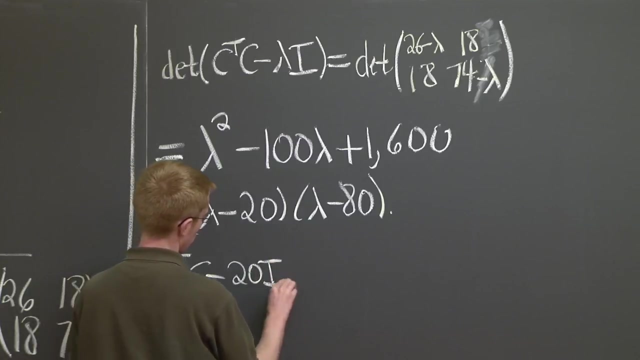 but you'll see, you get 1,600.. And this easily factors as lambda minus 20 times lambda minus 80.. Good, So the eigenvalues are 20 and 80.. OK, now, what are the eigenvectors? Well, you take C, transpose C minus 20 times the identity. 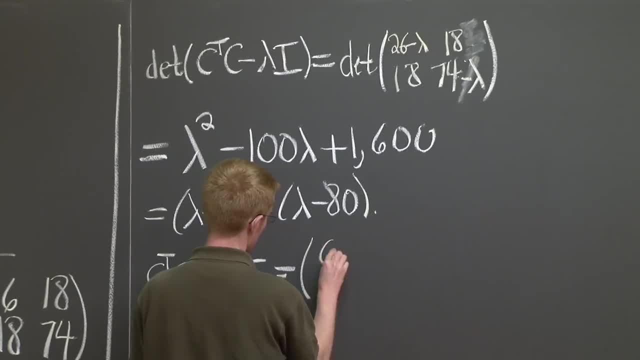 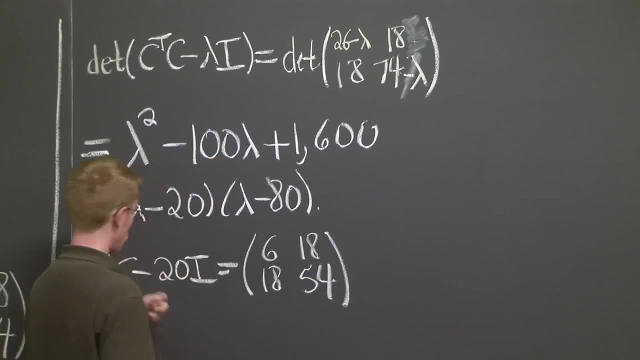 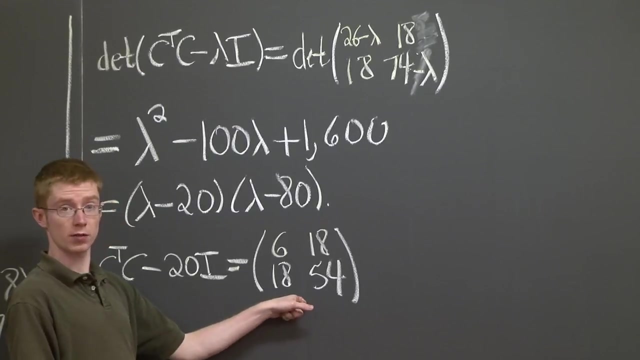 and you get 6,, 18,, 18, and 54.. To find the eigenvector with eigenvalue 20, we need to find a vector. OK, Let's find a vector in the null space of this matrix. Note that the second column is 3 times the first column. 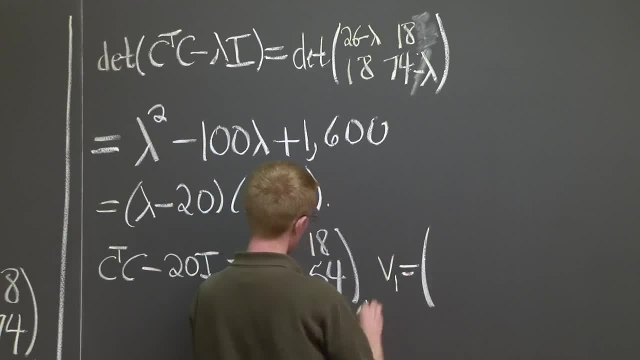 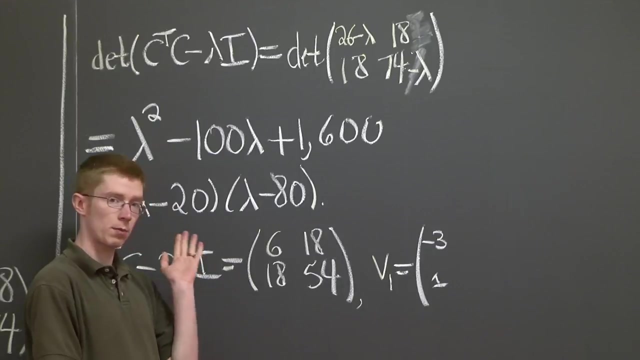 so our first vector, V1,. we can just take that to be well. we could take it to be negative 3, 1, but we'd like it to be a unit vector, right, Because remember the columns of V. 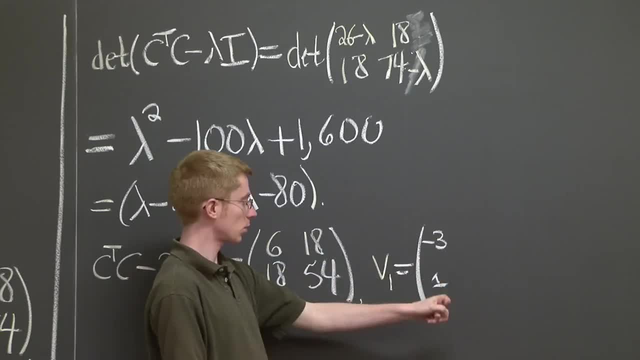 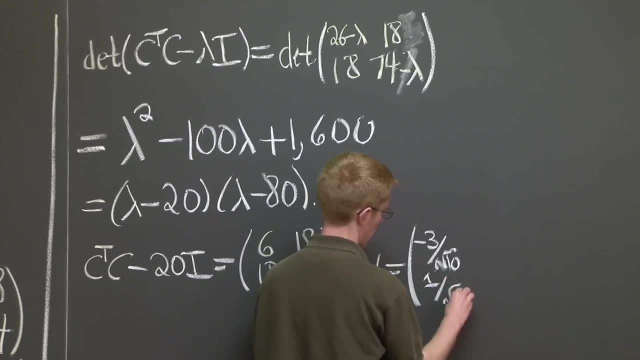 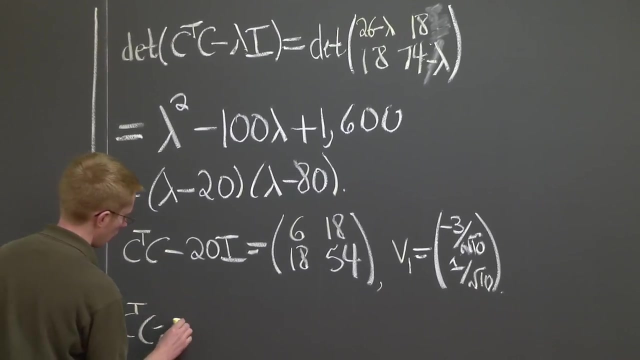 should be unit vectors because they're orthonormal. So 3 squared. So 3 squared plus 1 squared is 10.. We have to divide by the square root of 10.. Similarly, we do C, transpose C minus 80 times the identity. 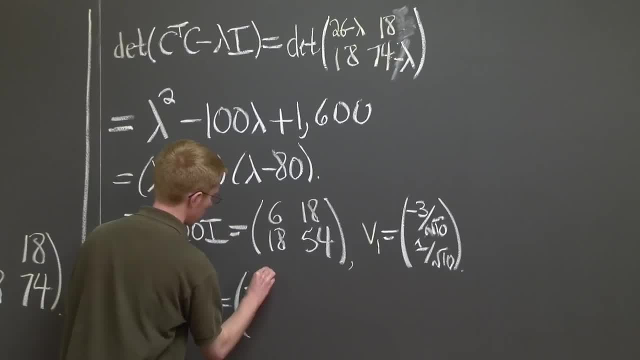 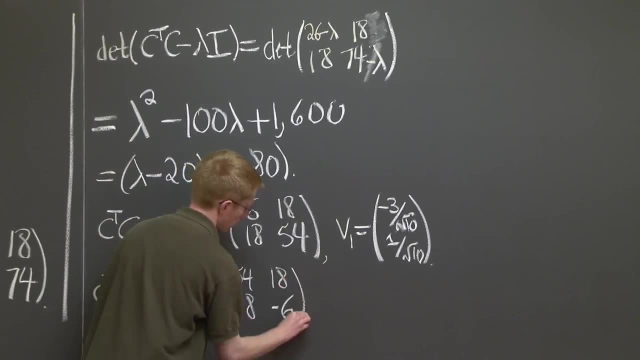 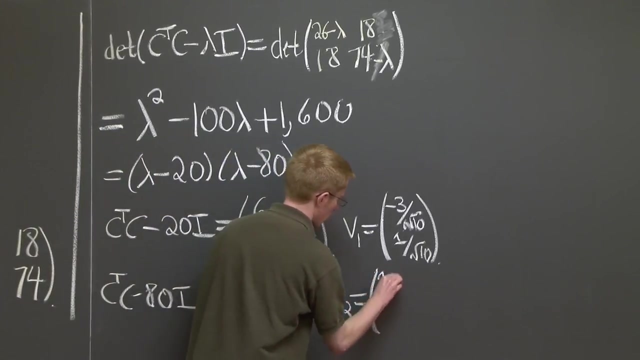 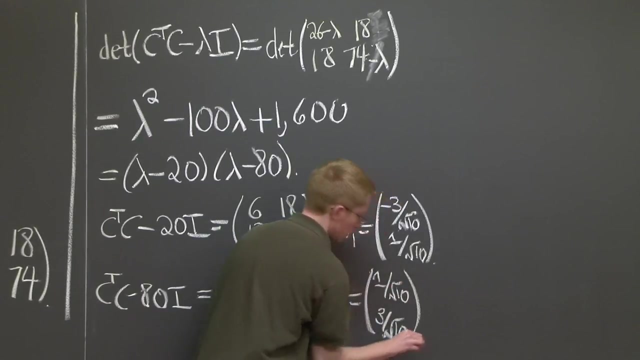 We'll get. what do we get? We get negative 54,, 18,, 18, and negative 6.. And similarly, we can find that V2 will be 1 over square root of 10, 3 over the square root of 10.. 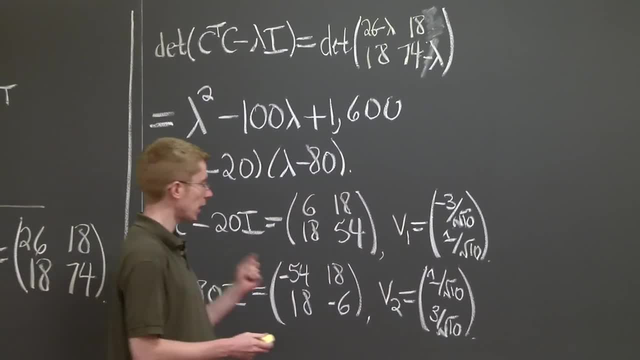 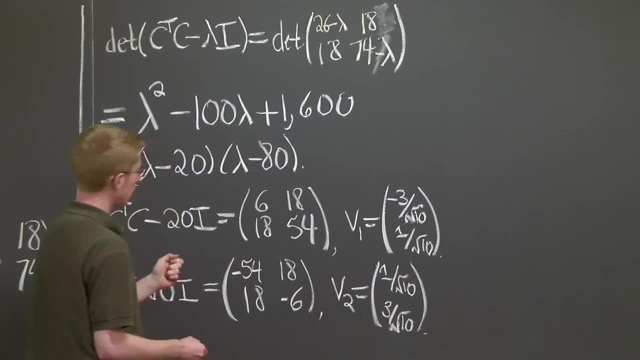 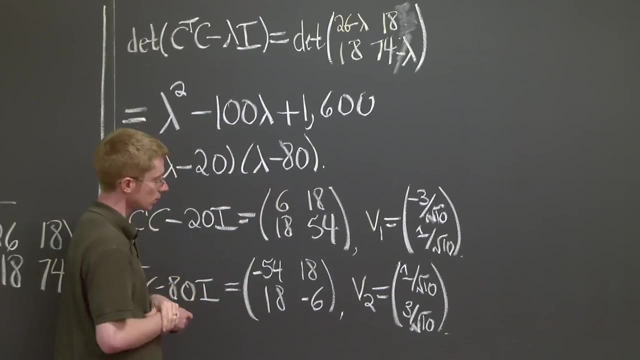 Great, OK, So what information do we have now? We have our V matrix, which is just made up of these two columns, and we actually have our sigma matrix too. right, Because the squares of the diagonal entries of sigma are 20 and 80.. 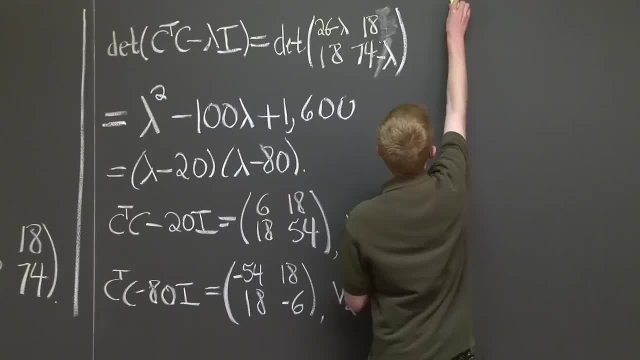 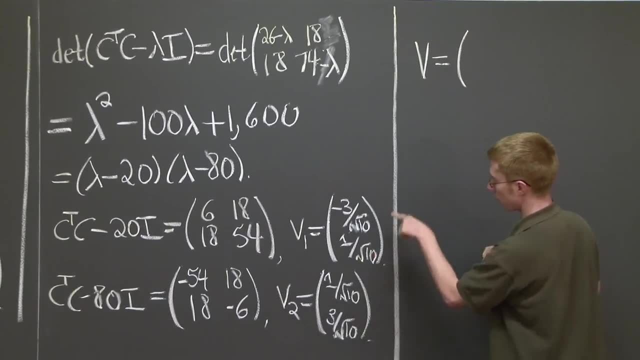 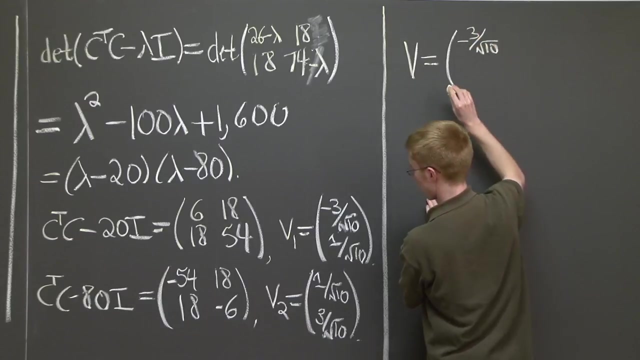 Good, So let's write those down. Write down what we have. So we have. V is just equal to. I just add these vectors and make them the columns of my matrix: Square root of 10,, 1 over square root of 10, 1 over square root. 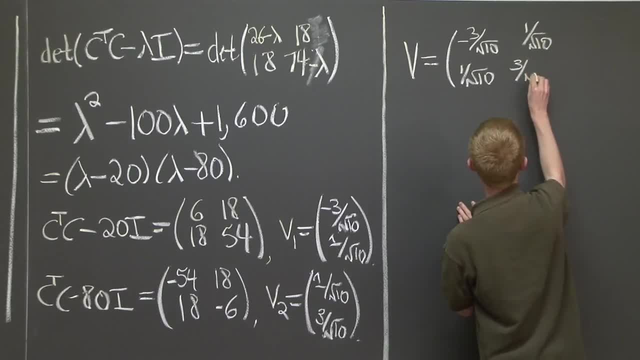 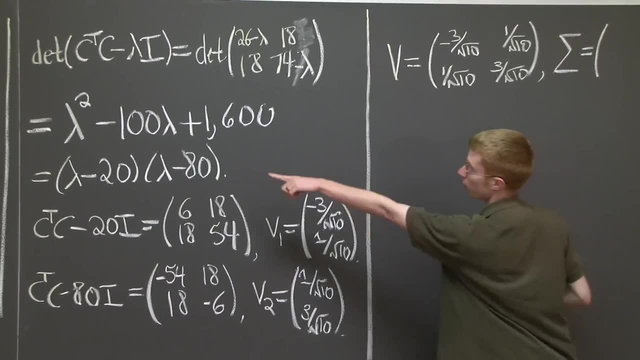 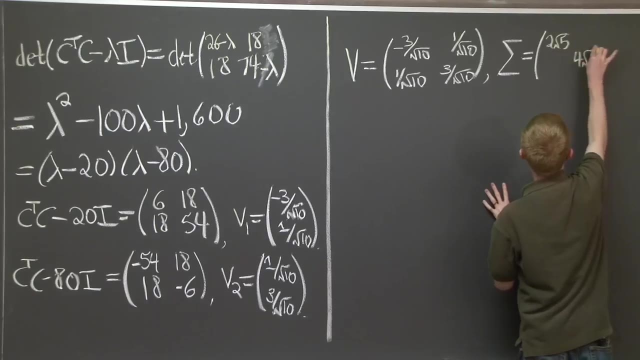 of 10, 3 over square root of 10.. OK, 3 over square root of 10.. And sigma, this is just the square roots of 20 and 80, which is just 2 root 5 and 4 root 5 along the diagonal. 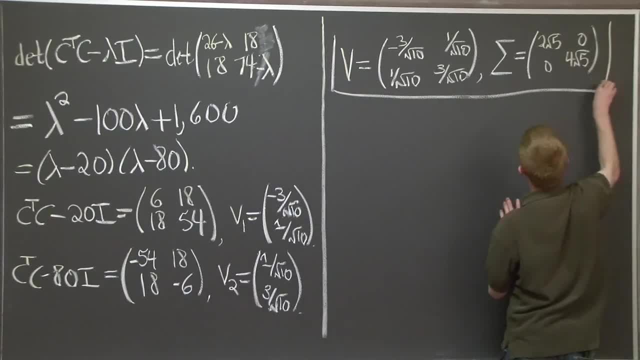 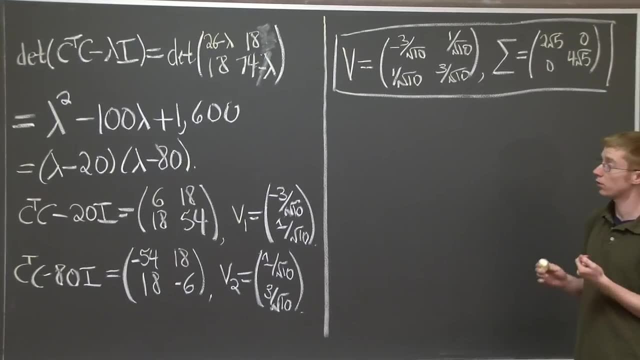 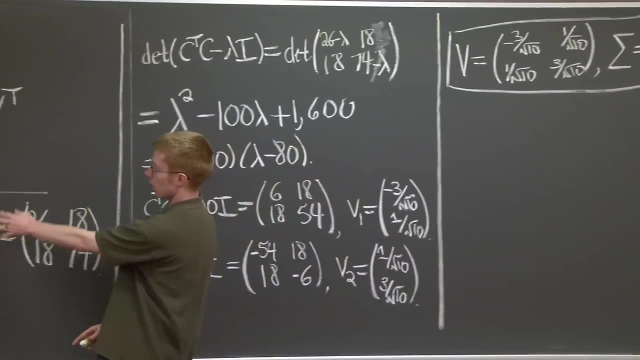 Squeezing it in here. I hope you all can see these two Good. So these are two of the three parts of my singular value decomposition. The last thing I need to find is U, And for that I need to use this second equation right here. 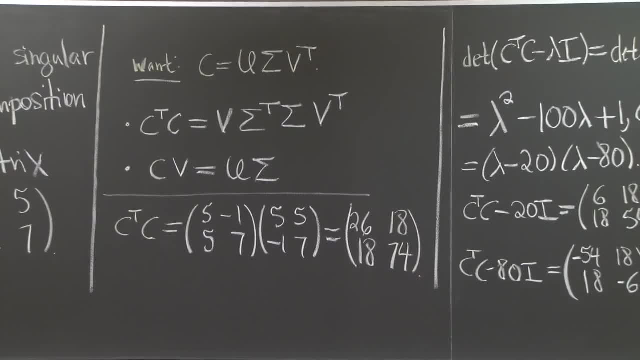 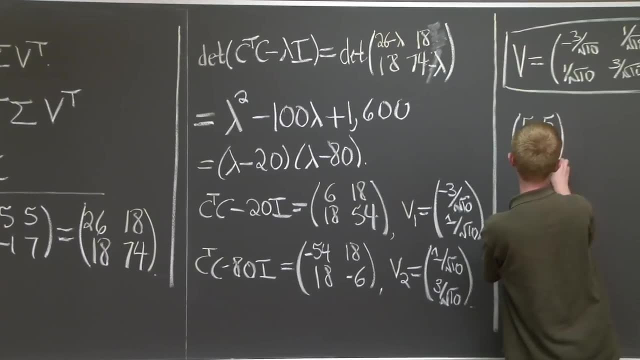 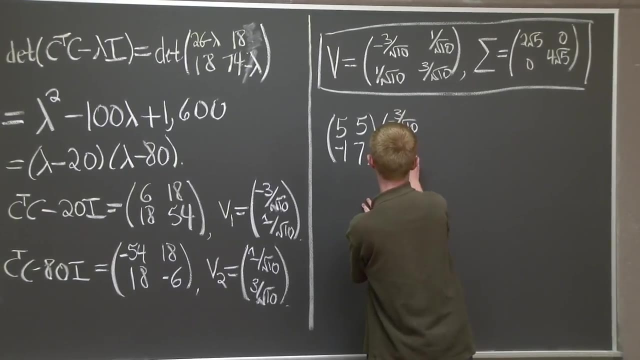 So I need to multiply C times V. OK, So C is 5, 5, negative 1, 7.. Let's multiply it by V: 1 over root, 10.. 3 over square root of 10.. 5, 5, negative 1, 7.. 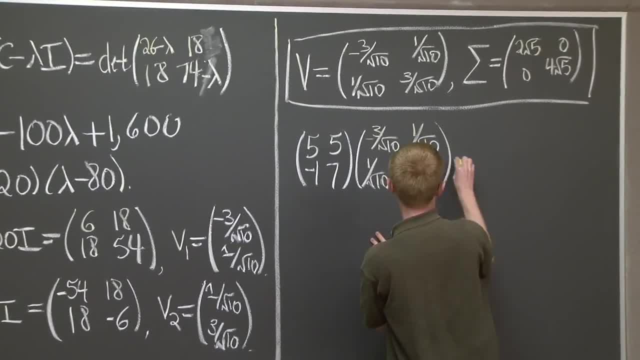 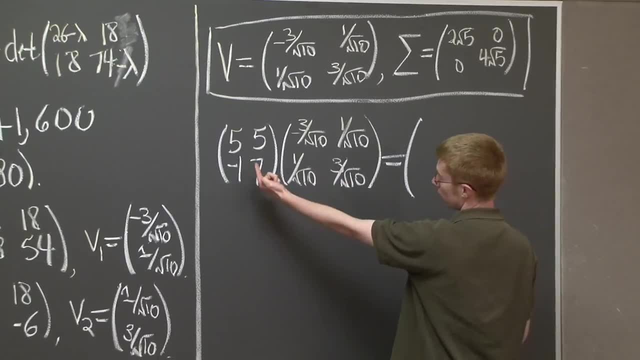 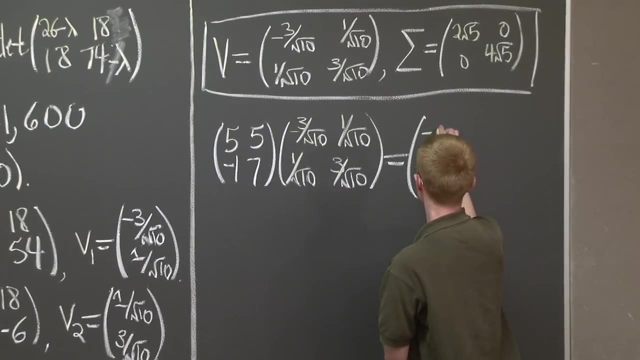 Let's multiply it by V: 1 over root 10.. 3 over square root of 10.. What do we get? Well, I'll let you work out the details, but it's not hard. here You get negative 10 over root 10,, which is just negative. 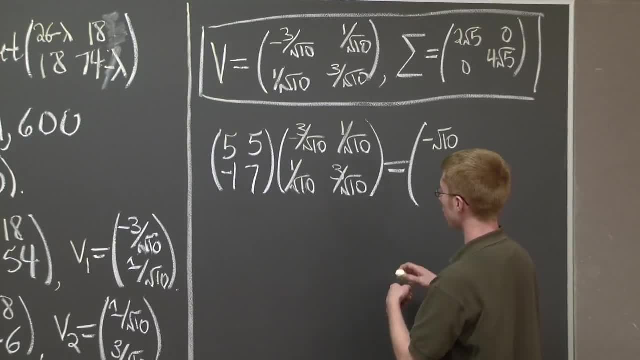 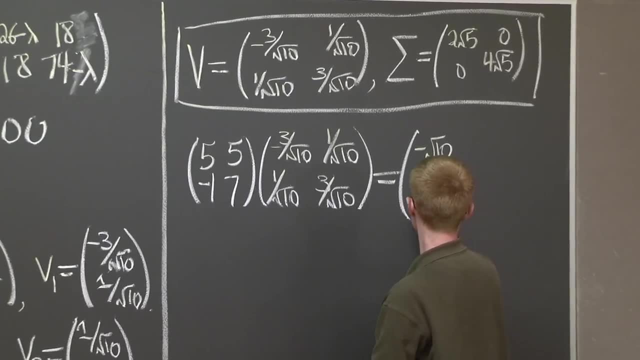 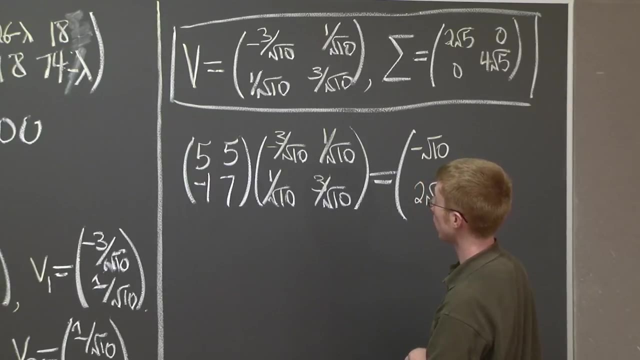 square root of 10 here. Then I just get 2 square root of 10.. OK, And then I get: 1 is 2 square root of 10, and I think I made an error here. Let me give me a second. 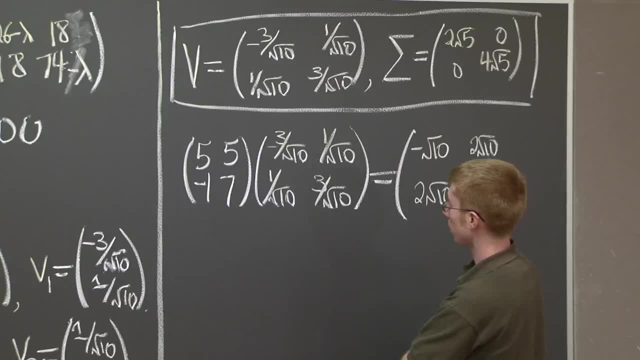 2.. Let me look through my computation again. The 2, 1 entry should be the square root of 10.. The 2, 1 entry should be the square root of 10.. Good, Yes, That's what I was hoping. 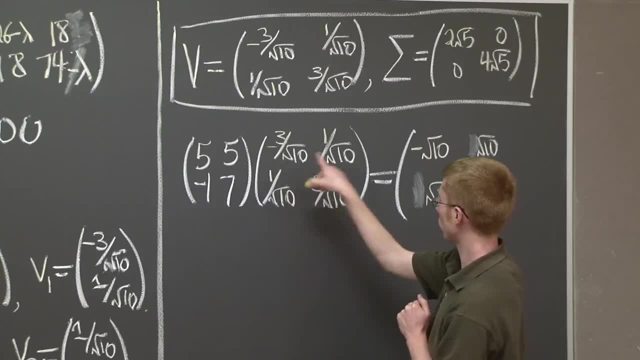 Yes, Because we get plus 15 is 20 over the square root of 10.. Oh yes, Sorry, I did it in the wrong order, right? So your recitation instructor should know how to multiply matrices. Great, Yes. 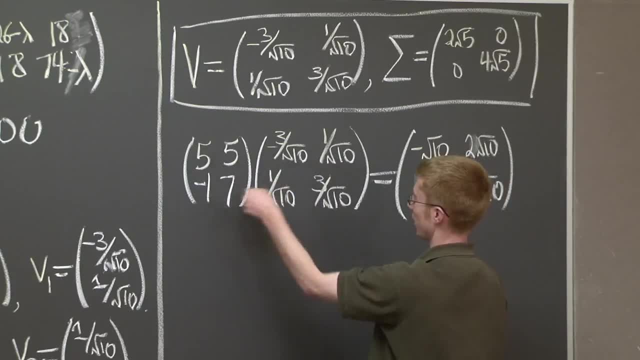 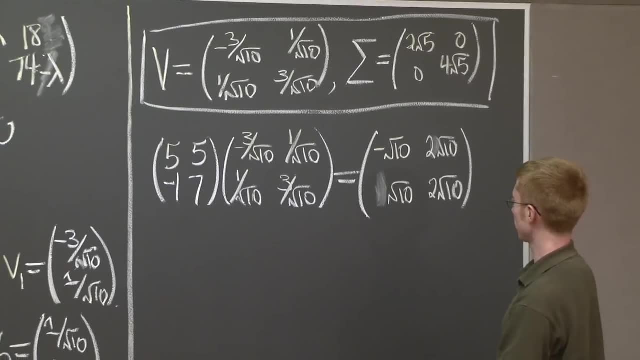 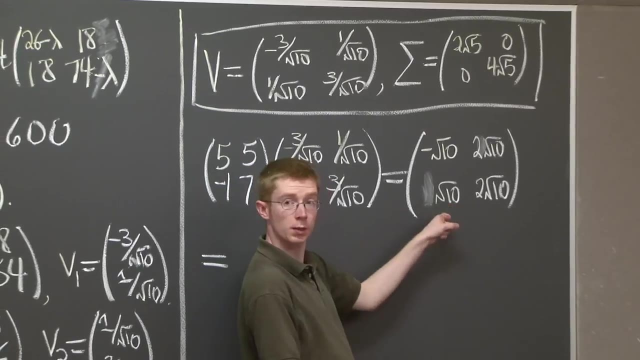 Thank you. You multiply this first, then this, then this and then this, And if you do it correctly, you will get this matrix here. Good, Great. So now I'd like this to be my U matrix, but it's actually U times sigma. 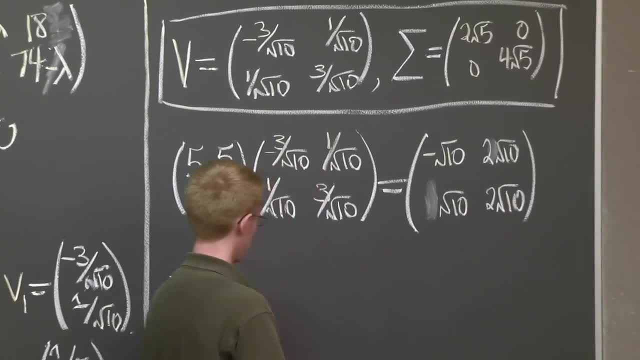 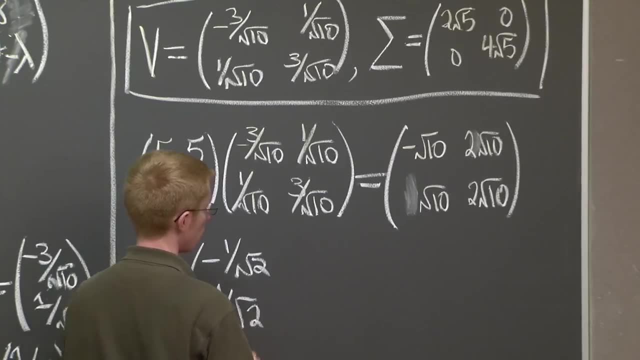 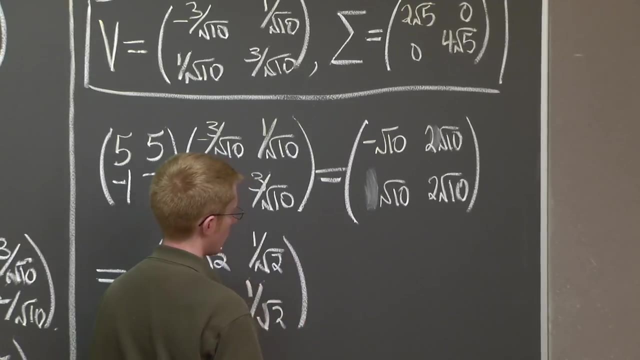 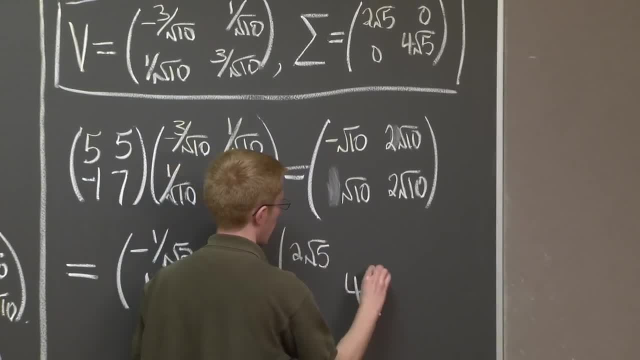 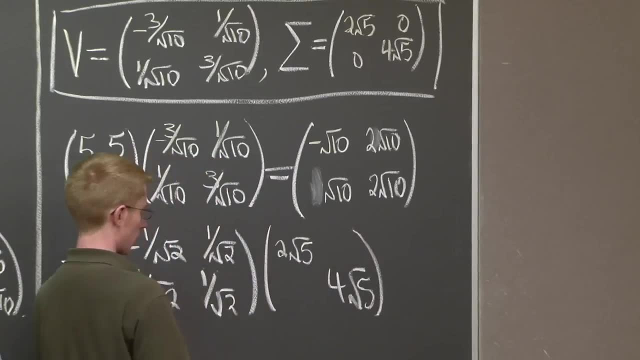 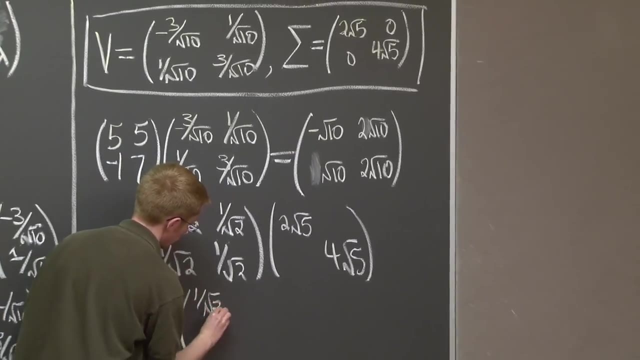 2 square root of 5,, 4 square root of 5,. and these constants are just what I needed to divide these columns by in order to make them unit vectors. Good. So now here's my U matrix: 1 over square root of 2,. 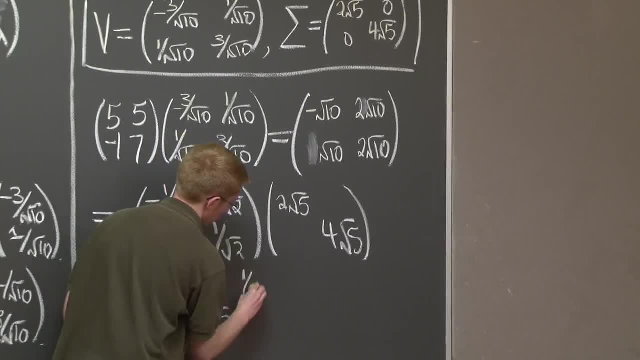 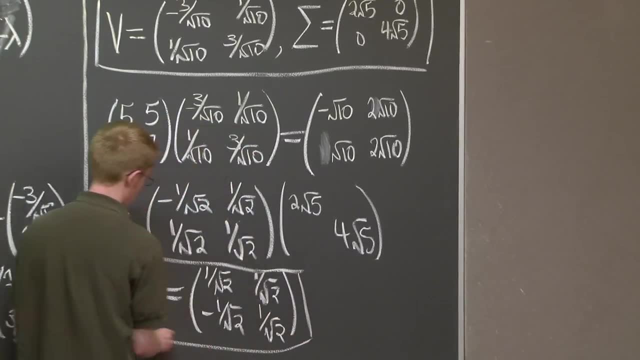 negative: 1 over square root of 2,, 1 over square root of 2,, 1 over square root of 2.. Good, So now I have all three matrices, U, V and sigma, And, despite some little errors here,